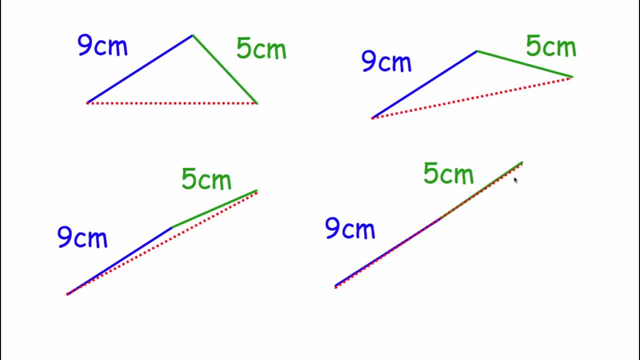 the length of that red line would be 14cm, but it can't actually be 14cm, so the length of this red line would be anything up to, but not including 14cm. So if we go back to our triangles whenever we've got our 12cm line, that would be possible, but our 20cm. 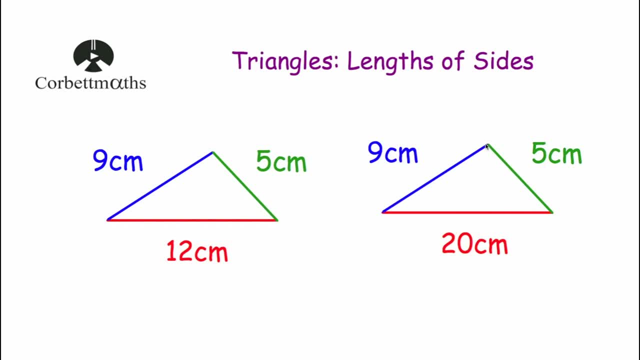 line wouldn't be possible, because even if it was a straight line, a 9cm line and a 5cm line, the 20cm would be far too large, so this triangle wouldn't be possible. Now let's have a look and see what happens whenever we make the angle between the two lines smaller. 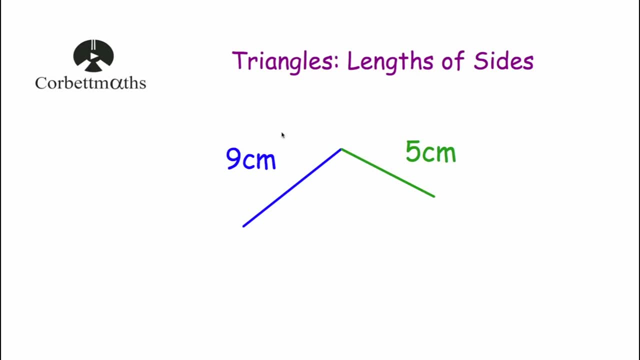 and smaller. So whenever we have our two lines, our 5cm line and our 9cm line, as we make the angle smaller between them, what happens is the length of the line joining the two ends of the lines would get smaller and smaller and smaller and smaller also, So it gets smaller. 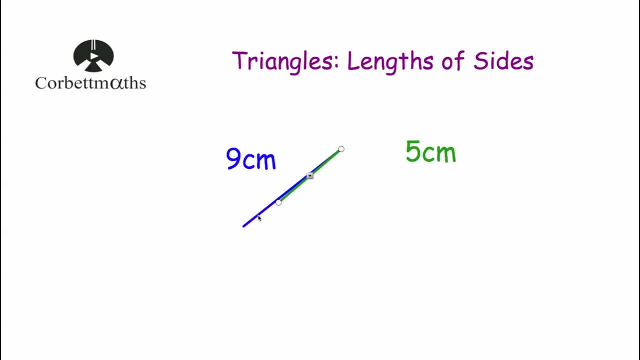 up until the point it's just before being on top of the other line, and then that would be the smallest possible. but then, once it's on a straight line, then it wouldn't be a triangle anymore. So let's have a look and see. So if we make the angle smaller, then 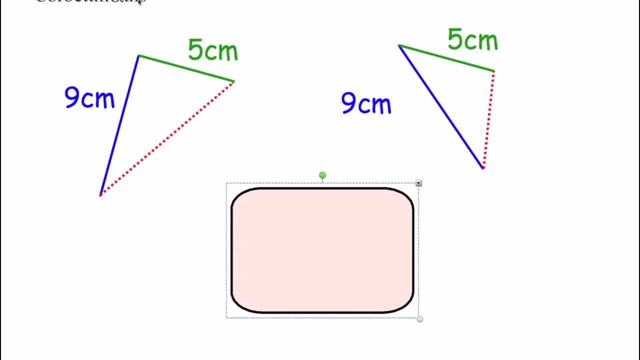 the red line gets smaller, and then if we make it even smaller still, then it would be the length of the third side of the triangle would be even smaller, but then it wouldn't be possible to have them on a straight line. So the length of this red line would be anything. 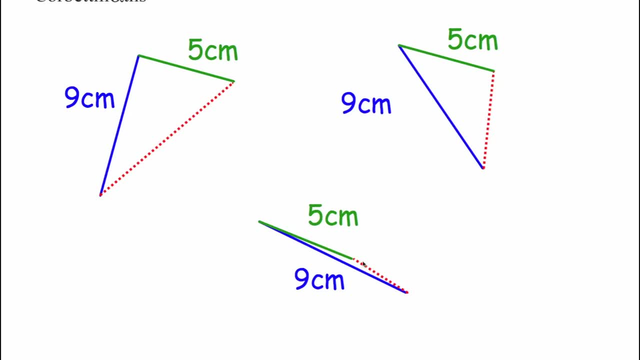 that is bigger than 4cm. It couldn't be 4cm because that would be a straight line, but it would be maybe 4.1cm and so on. So in terms of the lengths of the sides of the triangles, so what we've just found out, 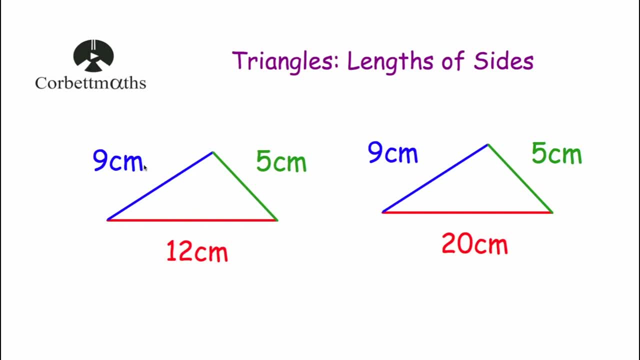 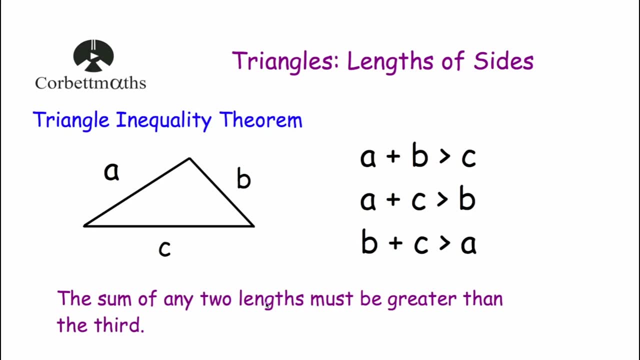 is that the length of the third side of the triangle has to be less than what you get whenever you add the other two sides together, and that gives us what they call the triangle inequality theorem. Now, I've never actually learnt this as a triangle inequality theorem. 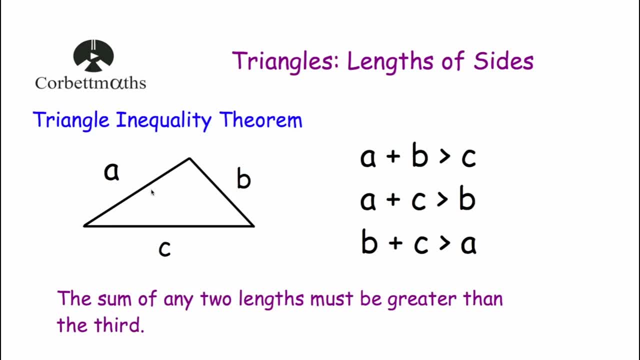 but it's common sense whenever you look at the sides of the triangles that you can't have a side that's far too big. But what it's saying is that whenever you add two sides of the triangle, it has to be bigger than the other side. So a plus b has to be bigger. 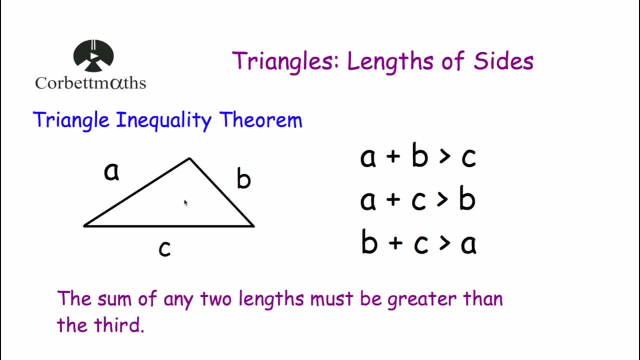 than c, a plus c has to be bigger than b, and b plus c has to be bigger than a. So the sum of any two lengths of the triangle must be greater than the third side of the triangle. Okay, let's have a look at some questions. So here we've got our triangles and we're 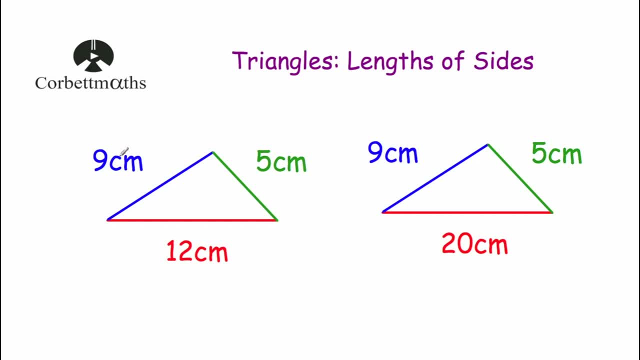 going to see which ones are possible. Well, if we add the two sides together we're at: nine plus five is fourteen. so that means that the other side has to be smaller than fourteen. so that would work. But in this one here, nine plus five is equal to. 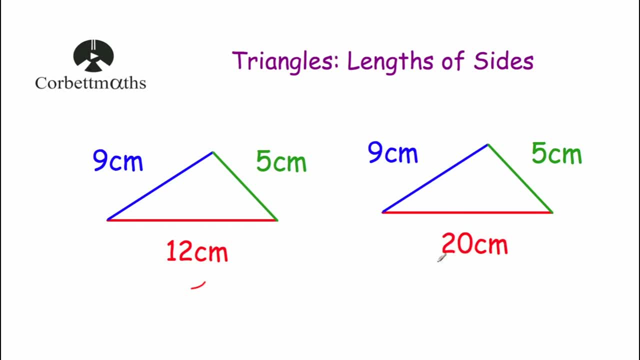 fourteen, so that means that this side has to be smaller than fourteen. it's twenty, so that's too big, so that triangle's impossible. Let's have a look at another pair of triangles. This triangle, we've got our sides and we've got five plus three. well, five plus three. 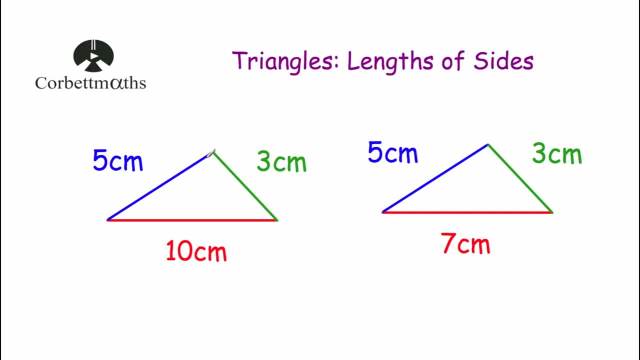 is eight, but this side's ten. that would be too big. So even if you put the five centimetre line and the three centimetre line in a straight line, the ten would be too large, so this triangle would be impossible. 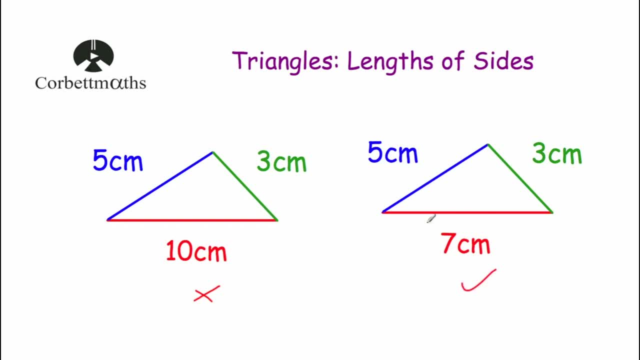 Five plus three is equal to eight. this side's smaller than eight, so this triangle is possible. Okay, let's have a look at another question. Okay, let's have a look at our next question. So the next question says the length of two. 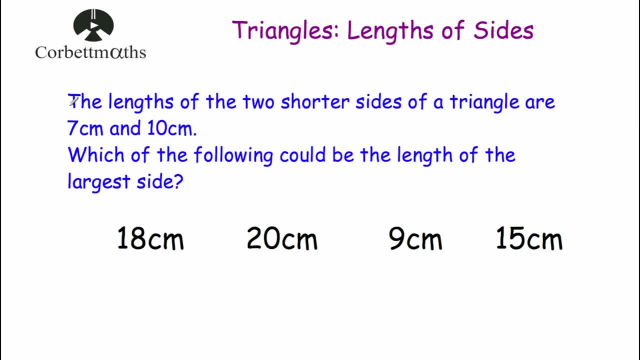 shorter sides of a triangle. so the two shorter sides of a triangle are seven centimetres and ten centimetres, which of the following could be the length of the largest side. So we've got our two shorter sides, so what I'm going to do is I'm going to add them together. 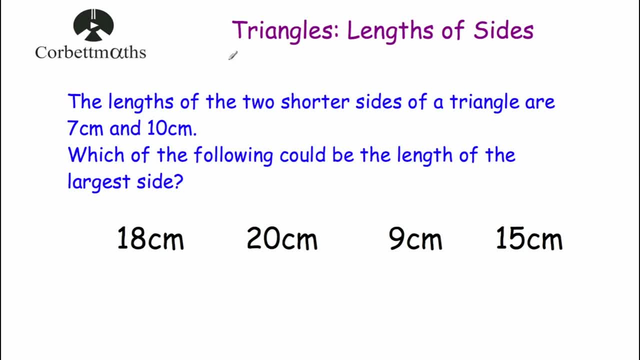 and see what the possible length for the largest one would have to be. So we've got seven plus ten. now, seven plus ten is equal to seventeen, so that means that the length for the largest side has to be less than seventeen centimetres, So it couldn't be eighteen centimetres, that's. 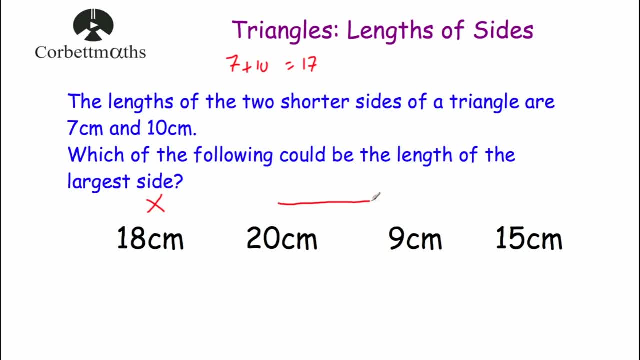 too long. If you had an eighteen centimetre line, like so, if you had a seven centimetre one and a ten centimetre one, they wouldn't reach each other. Likewise, the twenty centimetre one is too large as well. if you had a twenty centimetre line, the two, the seven centimetre, 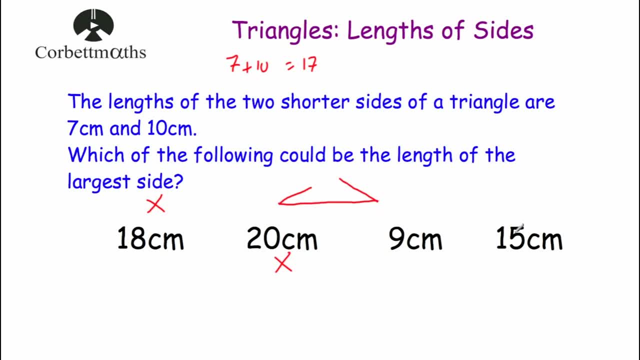 one and the ten centimetre one wouldn't reach each other. Now you've got to be careful here. we've now got two options Now. they're both less than seventeen centimetres, but let's read the question. The length of the two shorter sides: 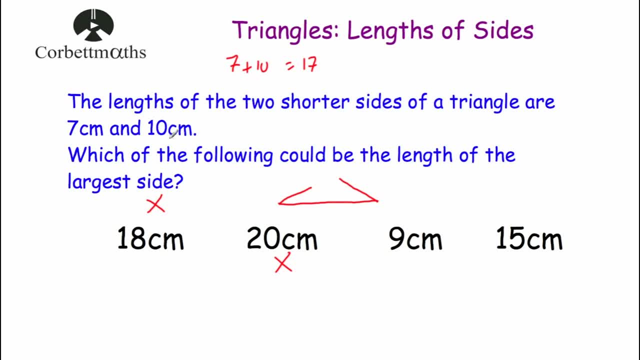 of the triangle are seven centimetres, So ten centimetres is one of the shorter sides, so nine couldn't be the length for the largest side, so it can't be nine centimetres And our final option is fifteen centimetres. 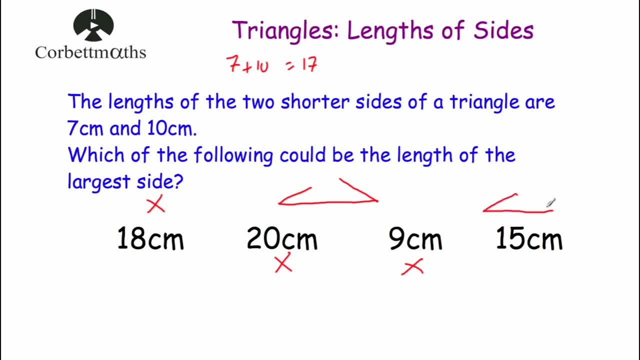 so if we had a fifteen centimetre line, you could use a seven centimetre line and a ten centimetre line and they would join up. so fifteen centimetres would be a possible length for the longest side of the triangle. 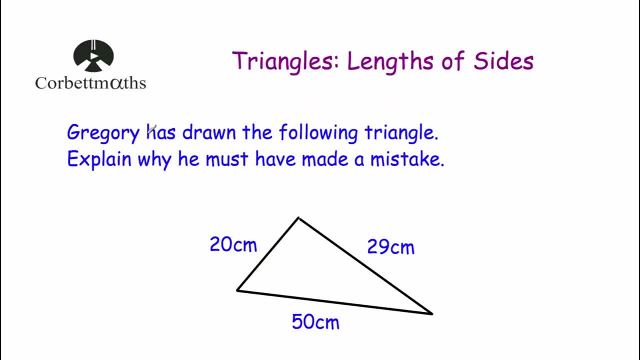 Okay, let's have a look at our next question. So our next question says: Gregory has drawn the following triangle: So we've got twenty centimetres, twenty-nine centimetres and fifty centimetres. Explain why he must have made a mistake. Well, if we have a look at the lengths of the 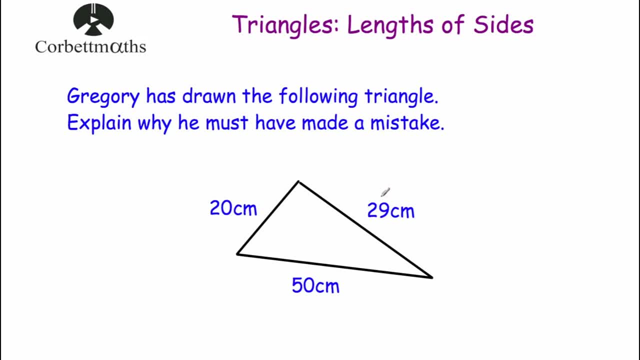 sides, if we look at the longest one. well, if we do twenty plus twenty-nine, twenty plus twenty-nine is equal to forty-nine centimetres. So that means that the length of the longest side has to be less than forty-nine centimetres. So that means that fifty can't be the length. 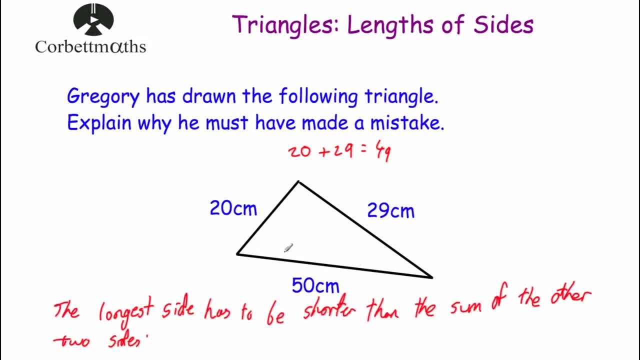 of this side. So we've just explained that, And that's it. I've just explained. the longest side of the triangle has to be shorter than the sum of the other two sides. So just remember, if you had a fifty centimetre line and you had a twenty centimetre line, 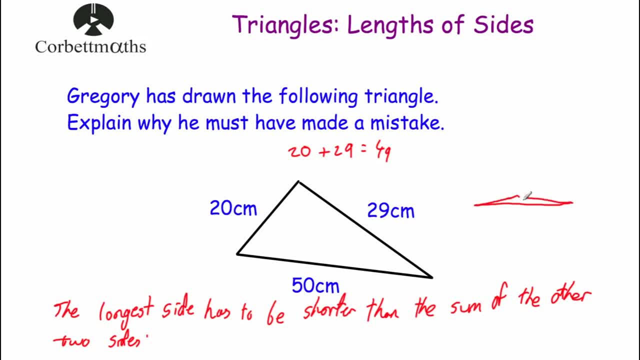 and a twenty-nine centimetre line. you could do this If you had a fifty centimetre line line. they wouldn't reach each other, they'd just be slightly short. so let's have a look at our last question. our last question says two sides of a 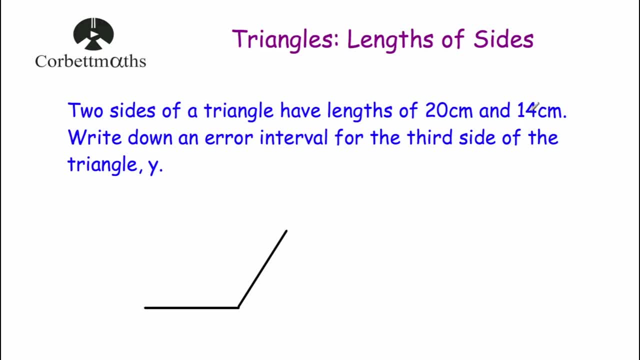 triangle have lengths of 20 centimeters and 14 centimeters. write down an error interval for the third side of the triangle. why so? if we've got two sides, let's call them 14 centimeters and 20 centimeters. let's consider what the 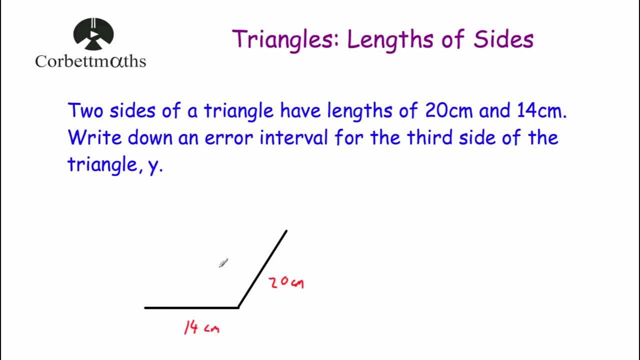 smallest possible length would be and the largest possible length for the other side, and in this question we're not told that this side is going to be the largest, and I just as two sides of the triangle. so let's consider the biggest possible length for that third side and the smallest possible length. so 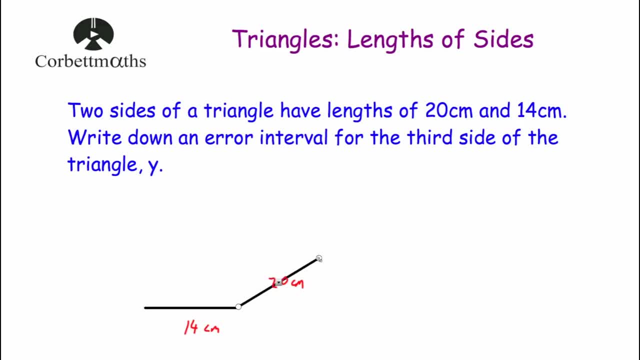 the biggest possible length. well, if we had this 20 centimeter line, we can increase the angle between them to whenever it's just before a straight line. if it was a straight line, then we would have a 34 centimeter line. that's not a triangle, so it has to be just slightly smaller than 34 centimeters. so 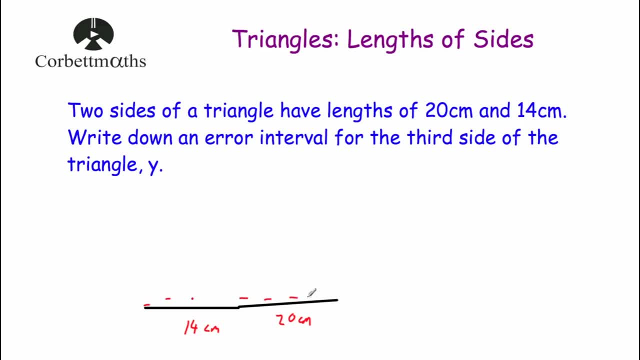 Y has to be the length of this side, Y joining them. Y would have to be less than 34 centimeters, so let's write that down. so Y. it has to be less than the sum of the silver two sides. so Y. the length of the third side has to be less. 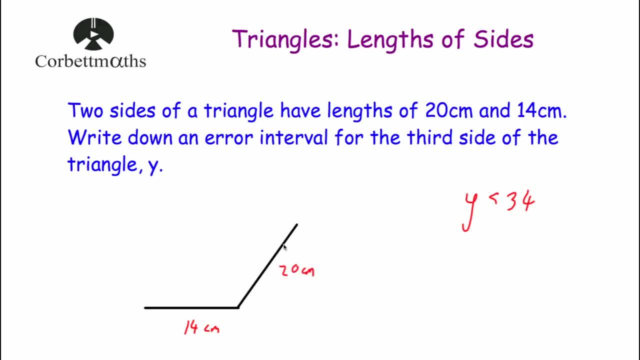 than 34 centimeters. so that's one part of the error interval. so now let's consider the smallest possible length of Y joining these two lines. well, if we make the angle between these two lines smaller and smaller and smaller, so we move, move the 14 centimeter line around to here. so just before being in a